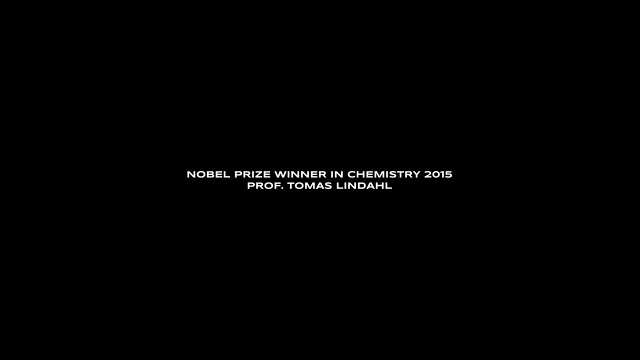 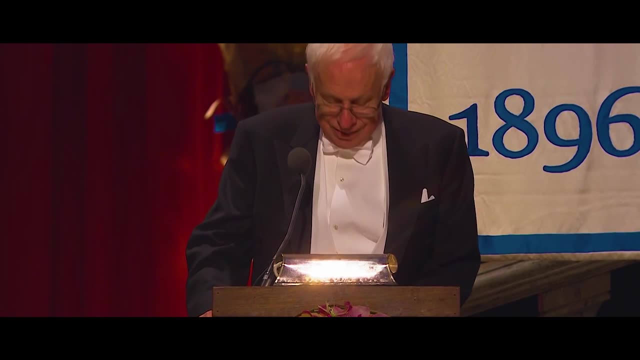 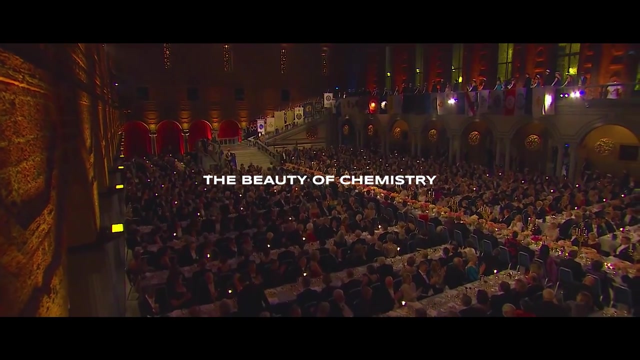 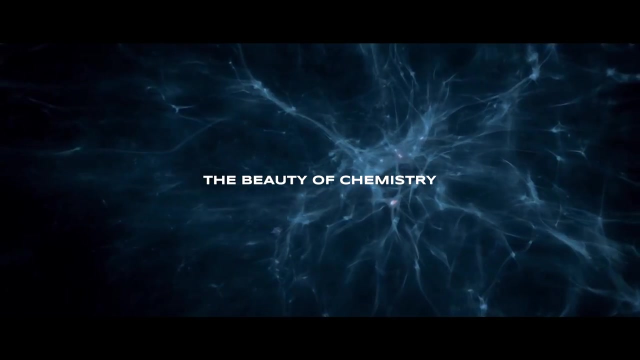 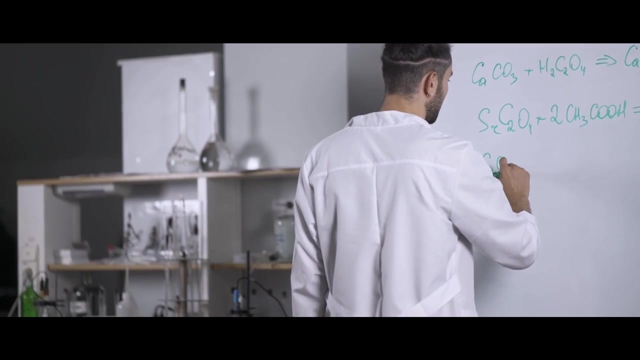 I did not like the teachers in the new school and, more to the point, the teachers did not like me. In fact, one of them failed me in chemistry. Chemistry is beautiful, Not because it has some fancy equations or beautiful and colorful chemicals. 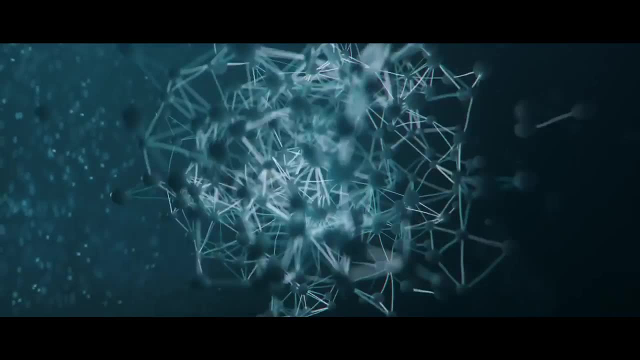 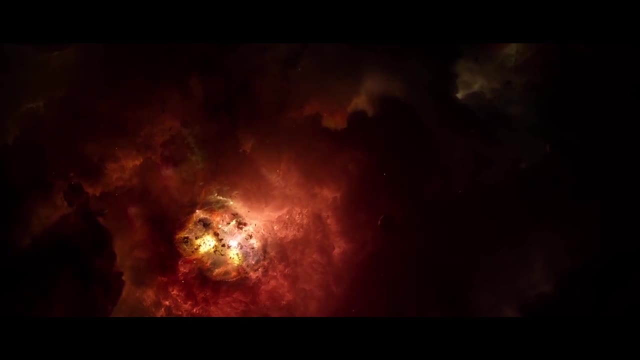 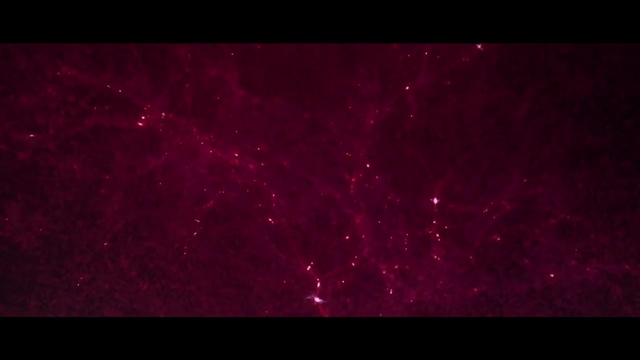 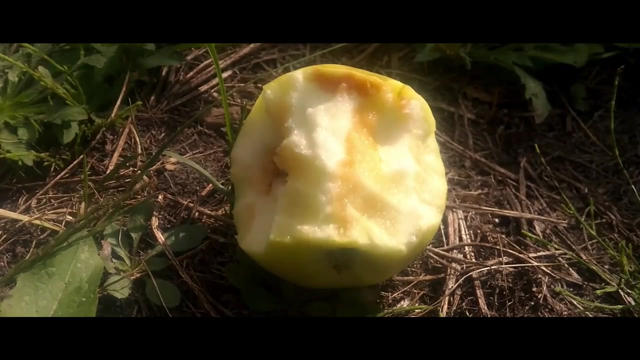 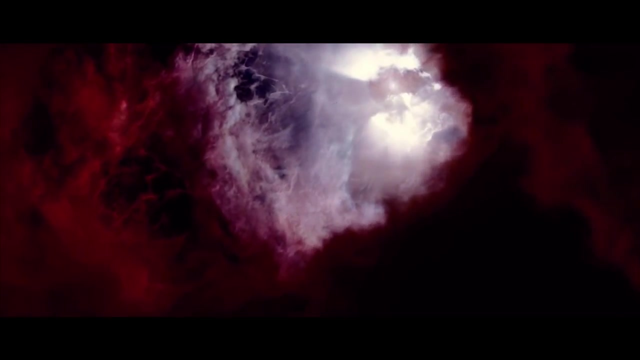 but because of its nature. If you think deeply, chemistry was born out of instability. Every single atom in this universe seeks stability. These reactions that we have in our books, everything that we see around, is the result of the instability in our universe. It's all due to uneven energy distribution. 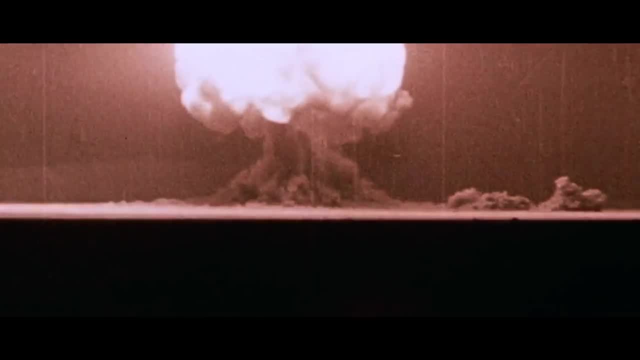 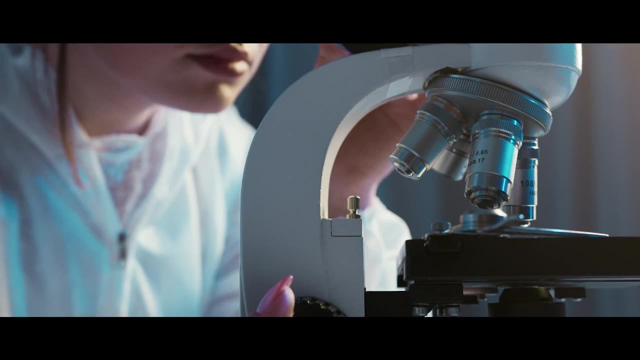 If you're the first person to do or see something, you're going to make a lot of mistakes. There's going to be a lot of failure because we're pushing for something that nobody knows about and we're trying to gain some understanding of it. 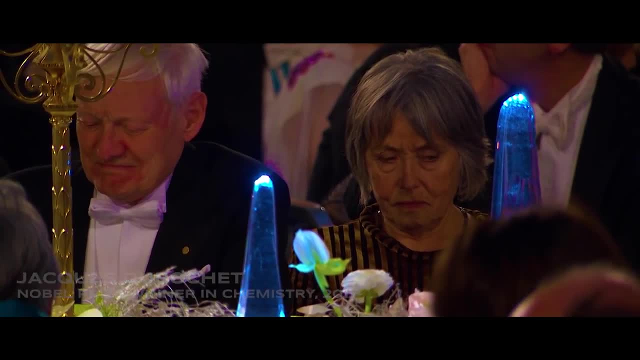 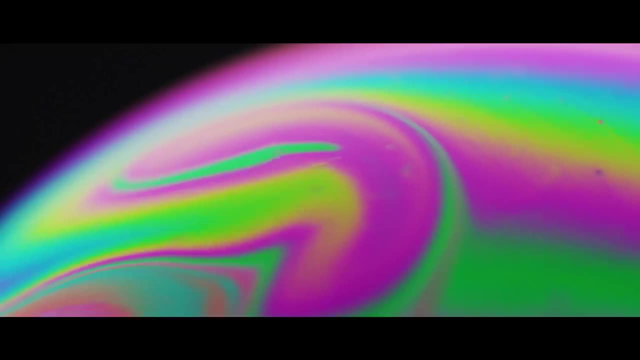 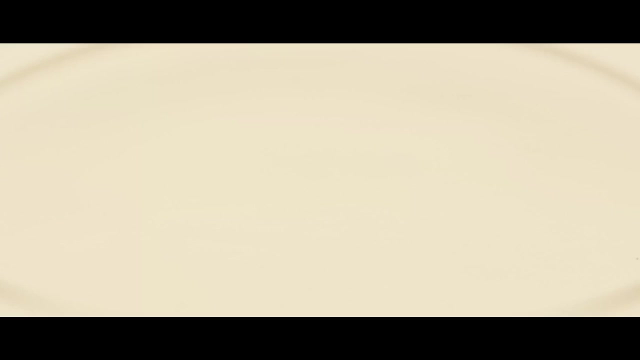 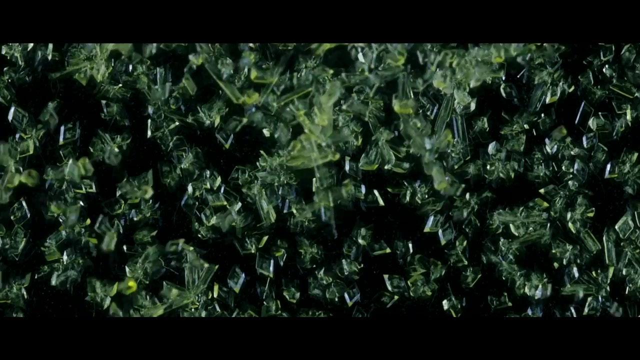 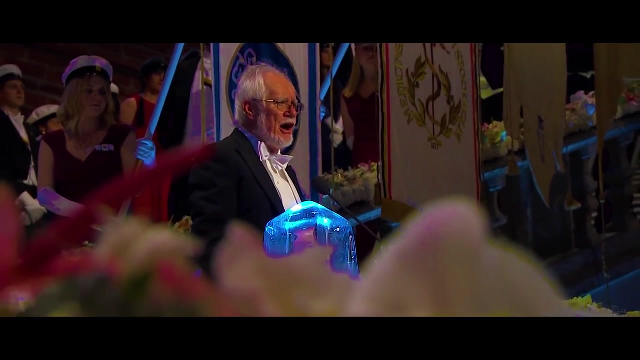 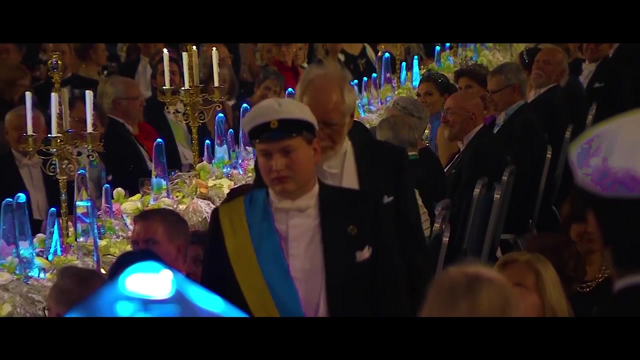 Chemistry is following the steps of Democritus. It deals about atoms: Study how the atoms are brought together or are not brought together, forming molecules or various complex structures. We three have never been good chemists. Nevertheless, we obtain a lot of good chemistry. 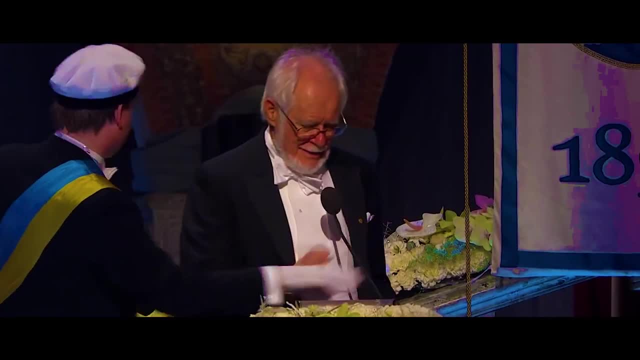 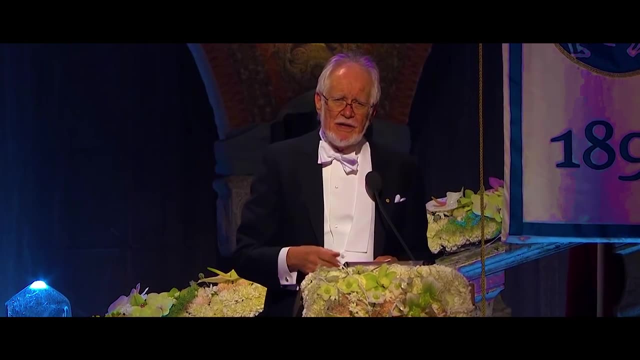 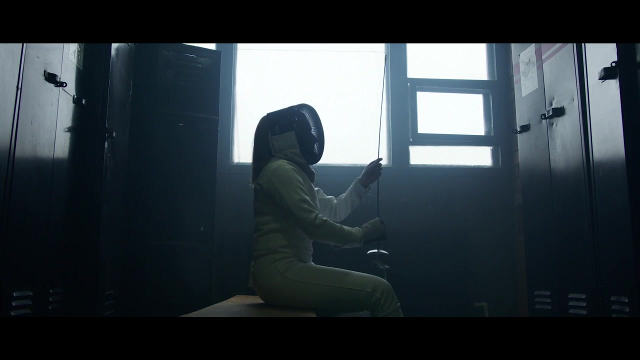 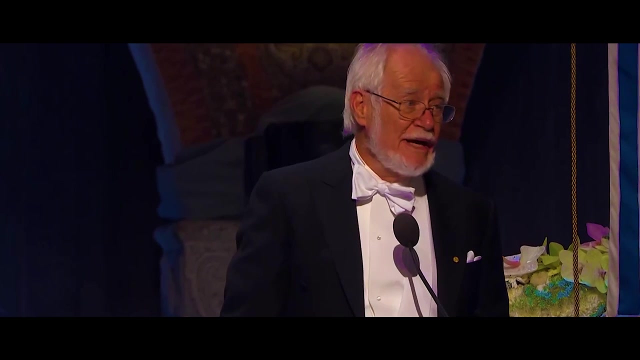 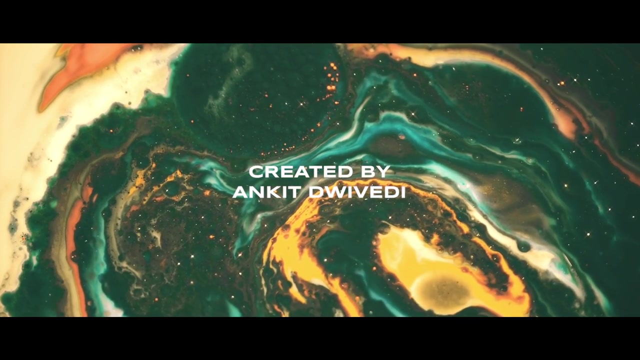 We've won a Nobel Prize in chemistry. Is this an illustration of the Peter Principle, which lets think that people reach their level of incompetence, Or perhaps it is simply a beautiful illustration of the unity of science? It's a beautiful illustration of the unity of science.